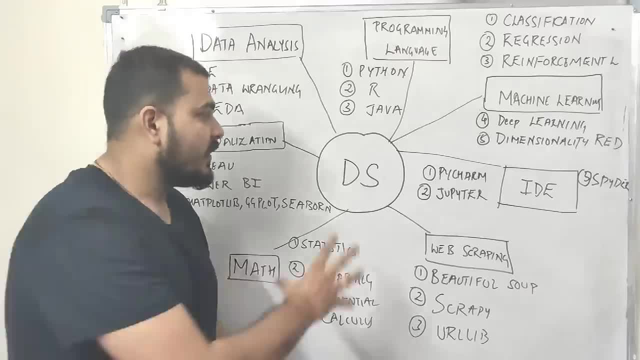 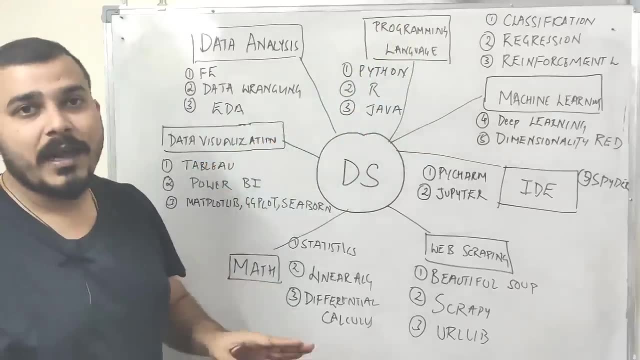 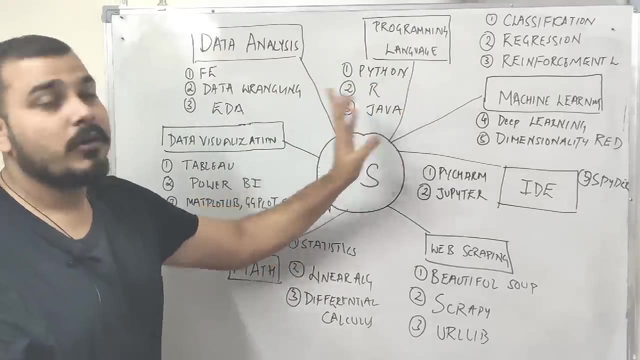 In the similar way. I'll basically be explaining you. So to begin with, in the center, I have data science. Now, in data science, you have to know various things, like at least one programming language. I would like to rank Python as first, then R and then Java, but I would prefer Python. 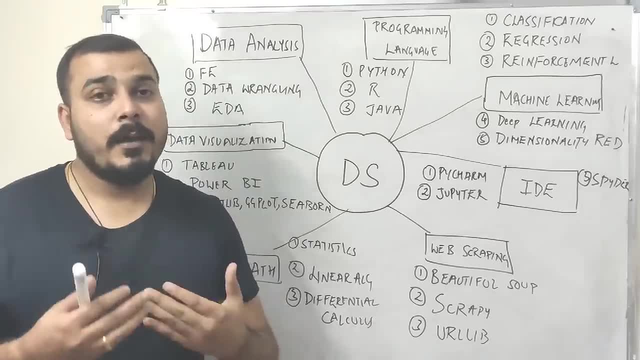 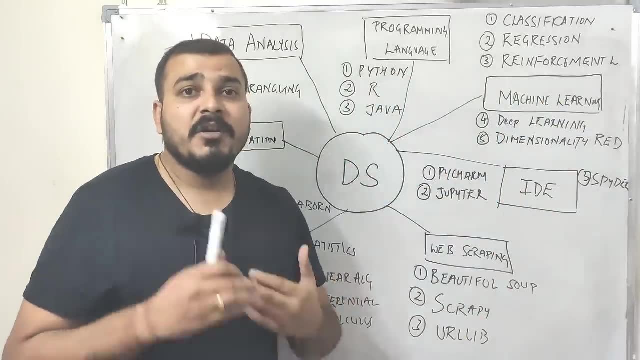 or R, because they have a lot of libraries and with the help of those libraries you can implement various machine learning algorithms. Then, when we consider machine learning in machine learning, there are various techniques, Like supervised, unsupervised machine learning technique, reinforcement machine learning. 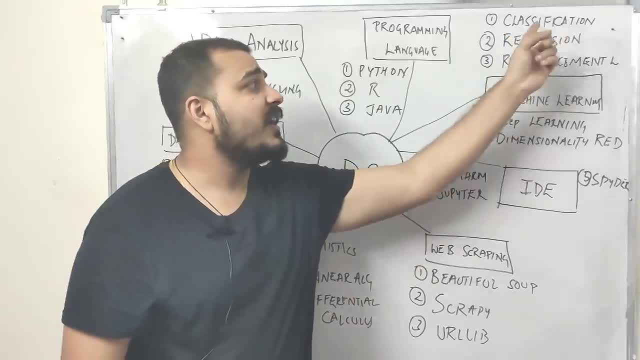 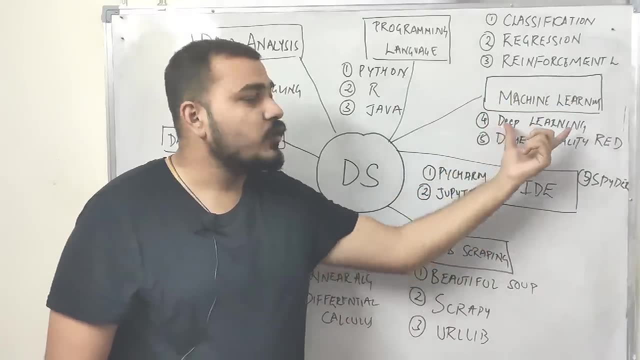 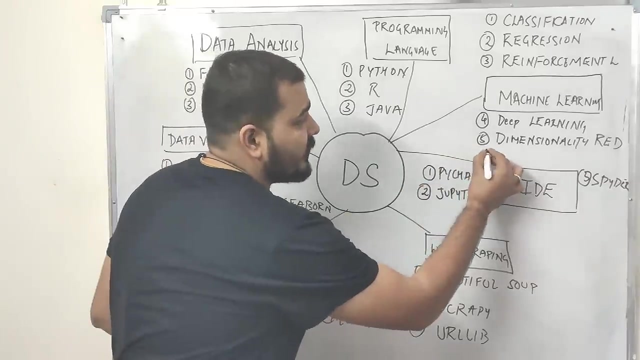 technique and many more. So in that you will basically be having problems like classification problem, regression problem, reinforcement learning and, as you know, that deep learning is a subset of machine learning. So I've mentioned over here deep learning and dimensionality reduction. Apart from that, we also have clustering algorithm. I would also like to specify clustering. 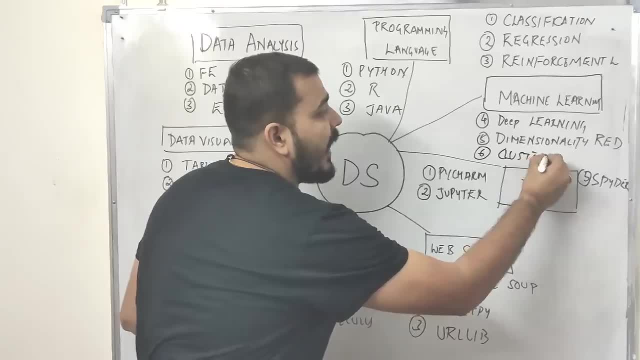 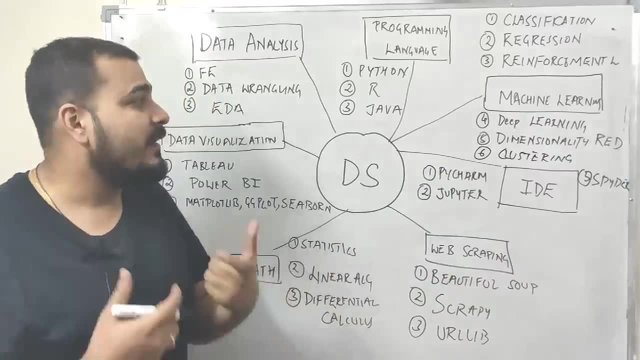 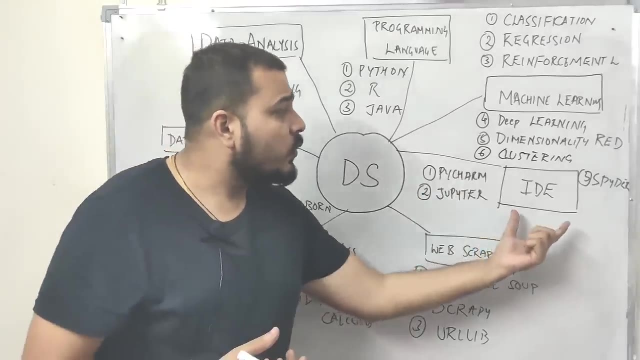 algorithm. So most of your problem statement actually revolves around this kind of scenarios only, And you basically be using machine learning for that, and deep learning is a subset of machine learning where you will be actually implementing those with the help of neural networks, And then after that you need to know some tools like IDE, And this IDE basically is: 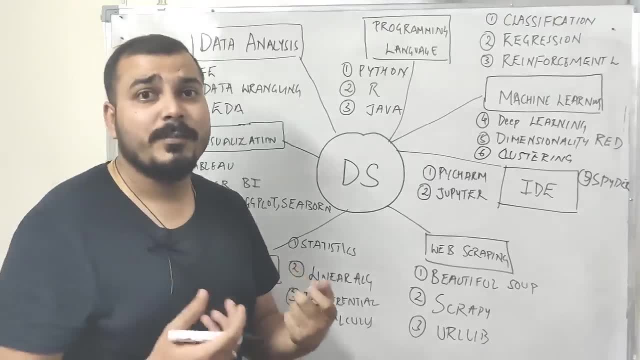 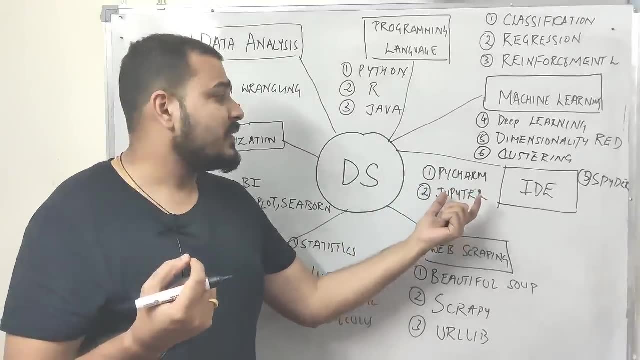 the integrated development environment, Like, basically, what kind of editor you are basically using for coding this? Python and R programming languages- and there are many. So for Python- I've just taken an example- There is a tool called spycharm, which is very, very nice. You. 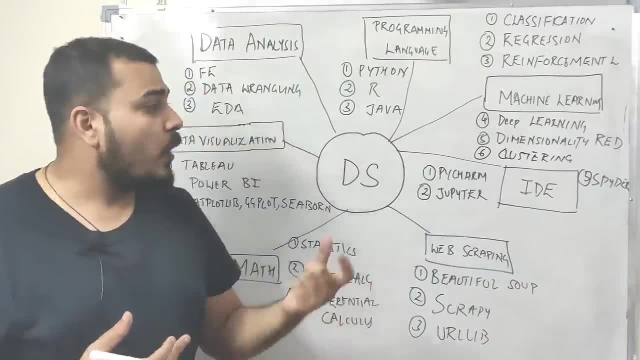 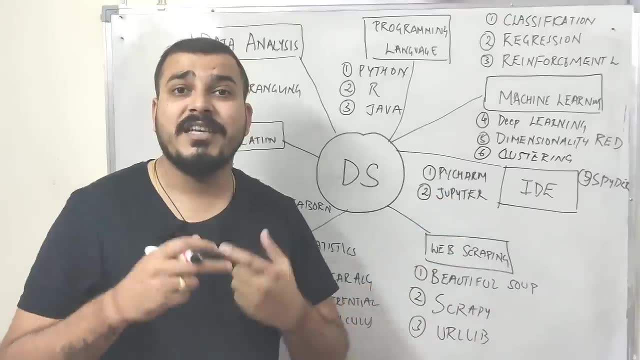 have Jupyter, You have something called a spider, now that all tools are basically present apart from that, for R programming language you have R Studio And for Python also, you have something called as VS Studio, Visual Studio. That is also a very nice tool, basically where 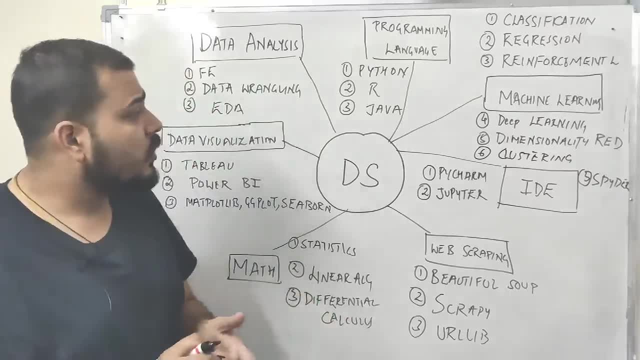 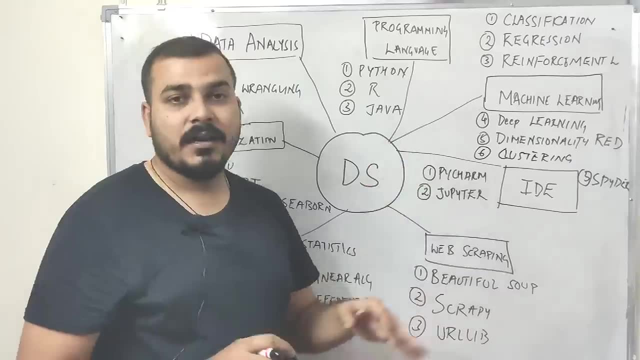 you can basically write, you can debug your code and do a lot of stuff, So you need to have a knowledge of one of the ideas. If you're going with Python, make sure that you have one of this. If you are going to R, you need to know how to work with R studio, because 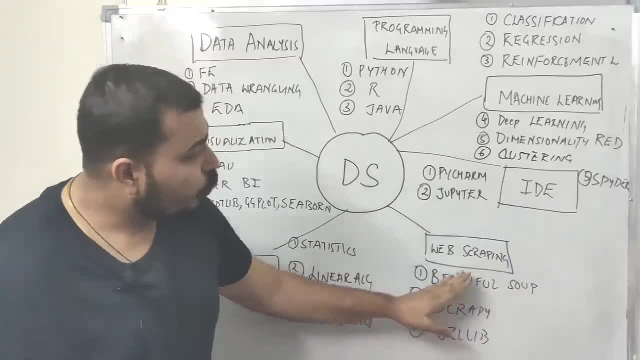 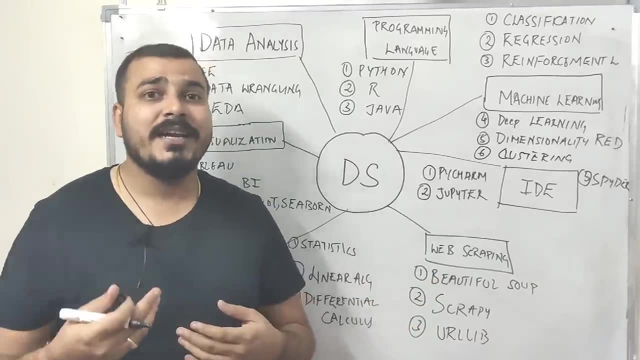 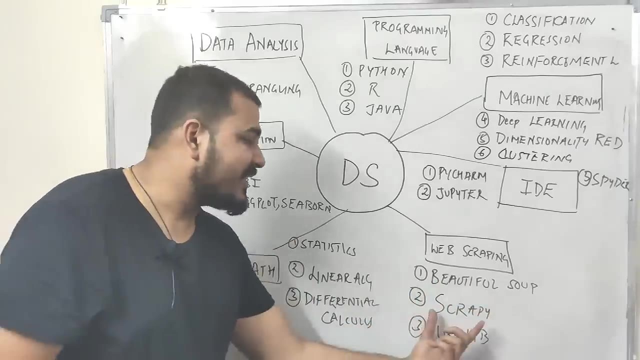 that is also a very good idea. web scrapping now, web scrapping it's not like you have to know extensively, but yes, in some of the scenarios where you need to collect data, you basically will be requiring this web scrapping and for that there are various libraries like beautiful soup, there is tool like scrappy, and 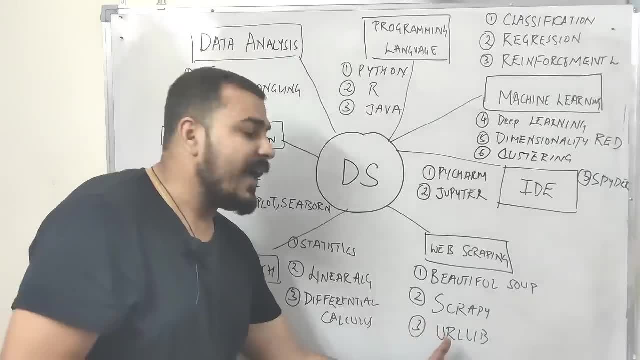 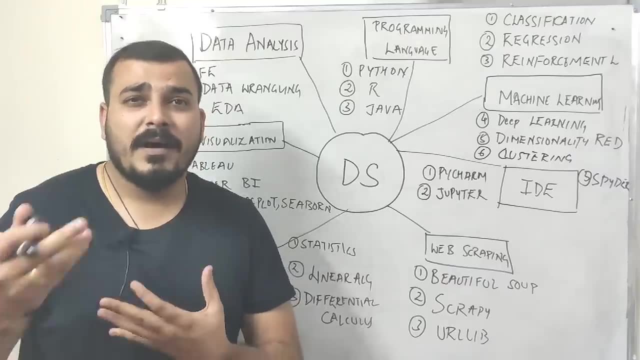 you'll also be using this another library, which is called as url lib, so this will actually help you to read some data directly from some url you know, in the form of json. apart from that also, you have various uh, your libraries in machine learning, like pandas and numpy. that will also help you to. 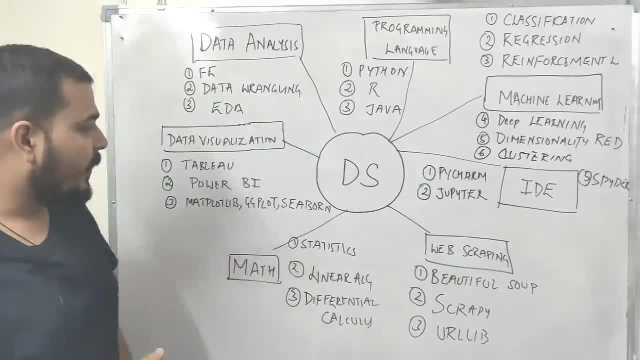 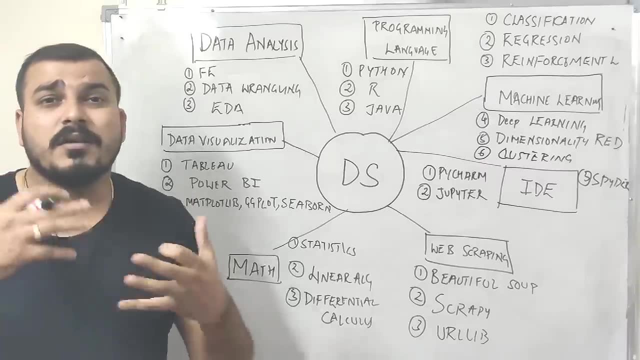 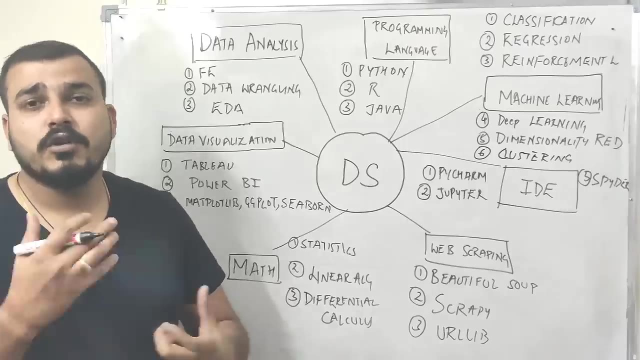 do it, you need to have some basic knowledge of web scrapping. apart from that, maths- as i said you yesterday also in my uploaded video i told you detailed what is the role of maths in data science. specifically, i would like to focus on statistics, linear algebra and differential calculus, because 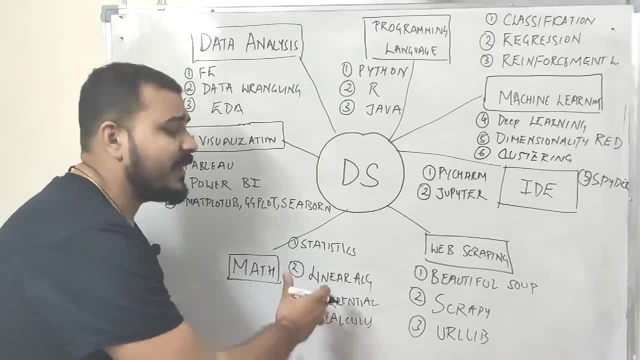 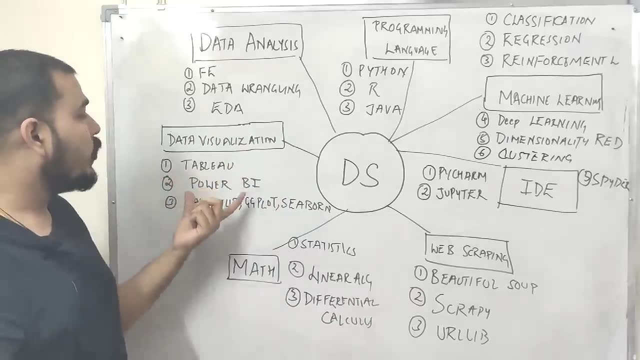 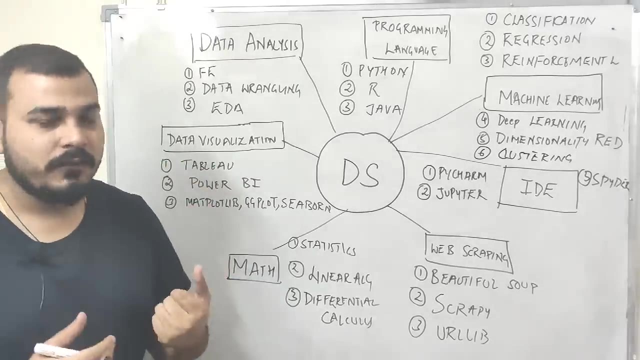 most of the algorithms. basic is basically on this particular concepts itself. then you should also need to know data visualization. now, data visualization: basically i have written tableau, power bi. so these are you know different tools where you will be able to do a lot of data visualization stuff apart from that in python and 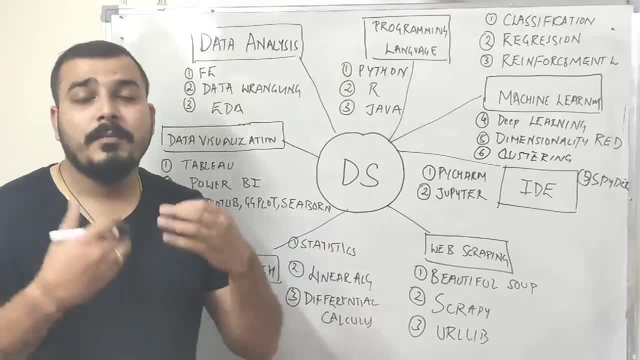 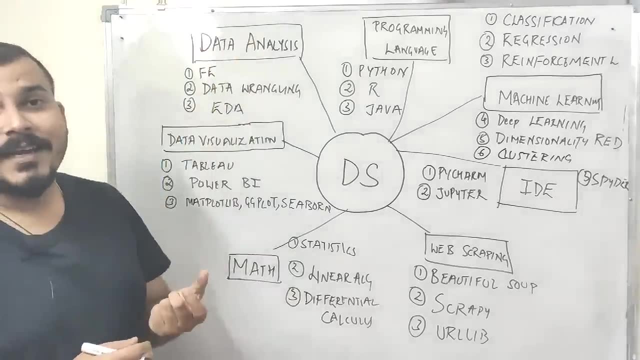 in r you have different libraries like matplotlib, seaborn, which will help you to actually do a lot of visualization with respect to your code that you are basically writing, and then you go to the data analysis stage also. this is also very important stage where you do feature engineering. 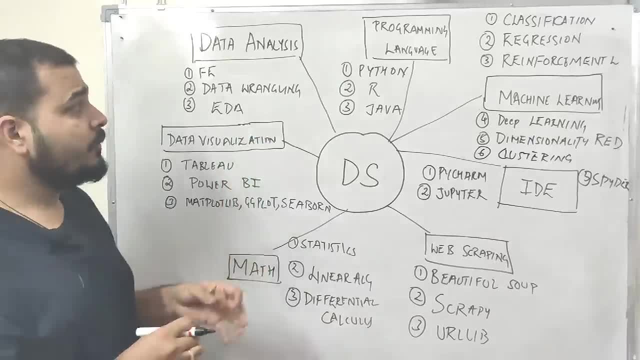 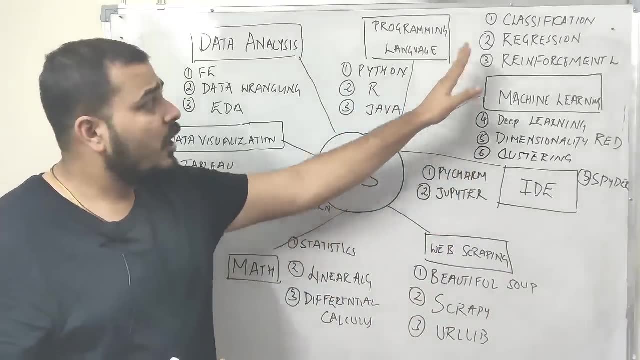 data wrangling, exploratory data analysis and a lot of things. now, from all these components that you have basically seen, you have to follow one one thing at least. so suppose in this you select a programming language. you should know all these particular algorithms and try to learn each and every algorithm, understand the maps behind them. 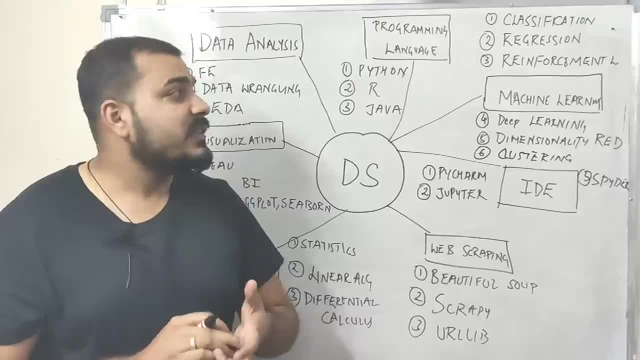 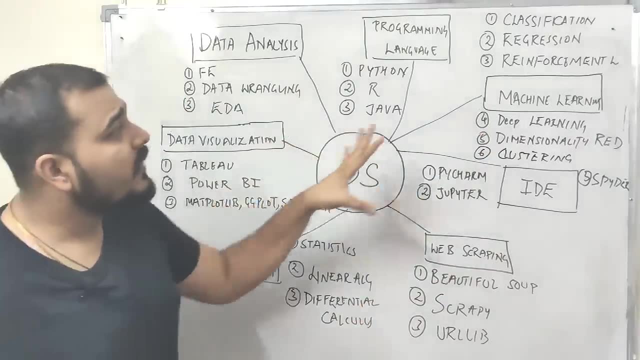 it is not like you have to just solve it somewhere, write it. no, just understand how this is basically getting implemented, because the main thing is your data science use case. based on this, you will be using different, different techniques. okay, suppose i have a use case where i need to predict the house. 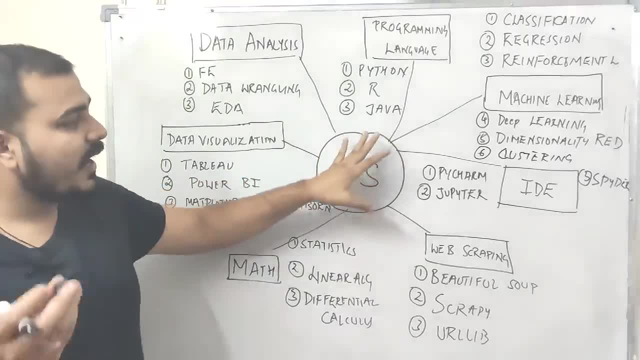 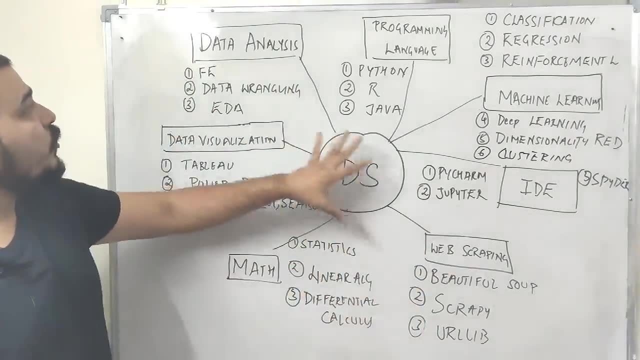 for a particular city, right? so what are the things that i'll require? first of all, i'll require data, right, i may take it through web scrapping. i may be dependent on some third-party apis right then. after that, i may do some data analysis on that particular data like. 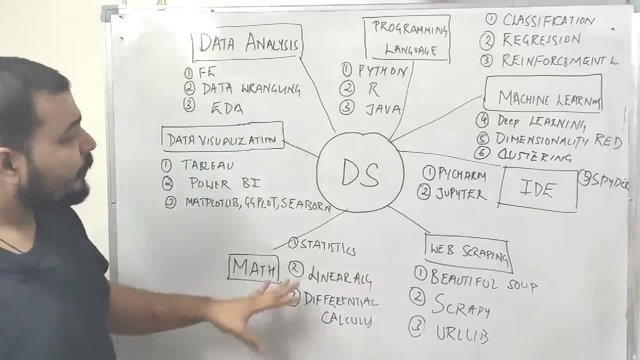 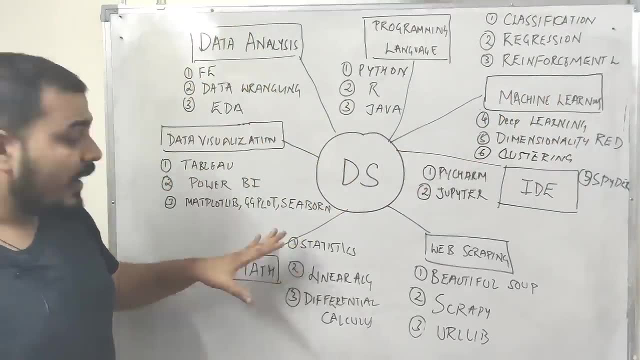 feature engineering, data wrangling, exploratory data analysis, and then, when i am selecting the algorithms, i will actually do data analysis along with that. i'll just see, uh, i'll just also apply some kind of maths to, and select a particular algorithm, perform that algorithm with the help of. 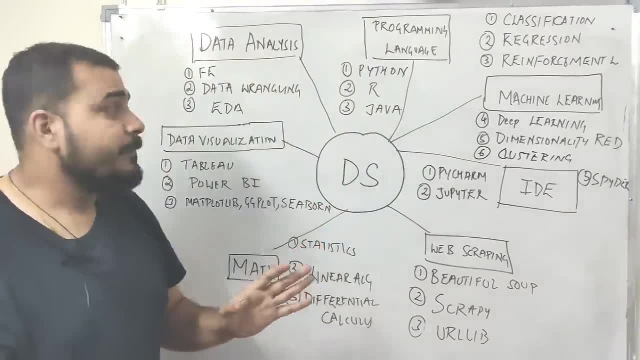 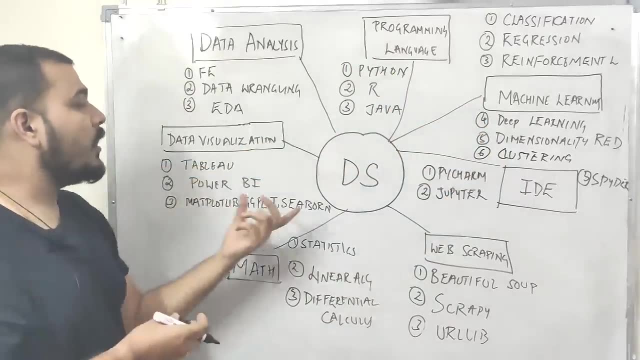 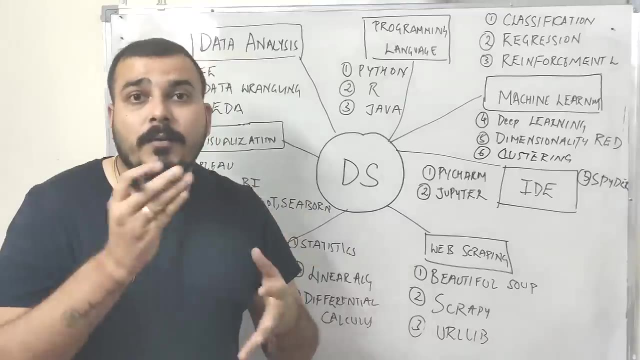 the techniques that i have learned in this and then i'll be able to implement that. apart from that, before implementing this particular machine learning algorithm, we may use some uh libraries like matplotlib c, bond tableau or power bi to actually understand about the data, how the data is basically distributed, what form the data is basically distributed, whether it is forming a. 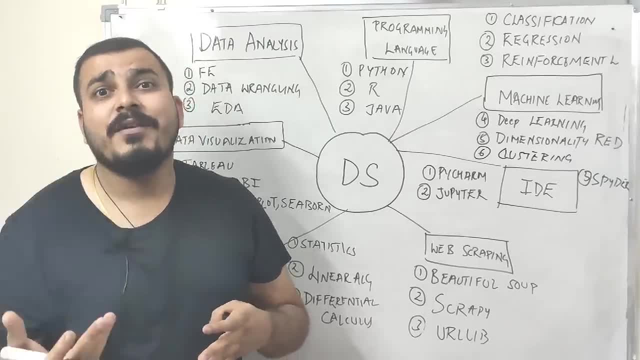 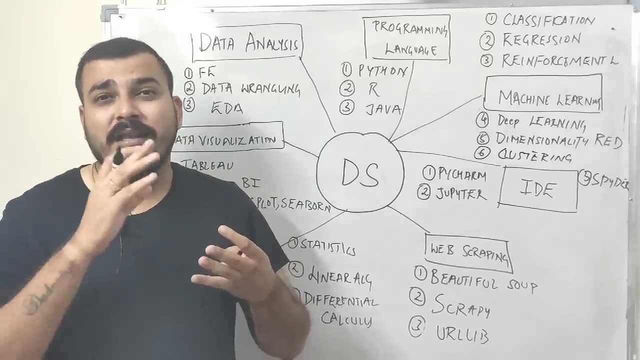 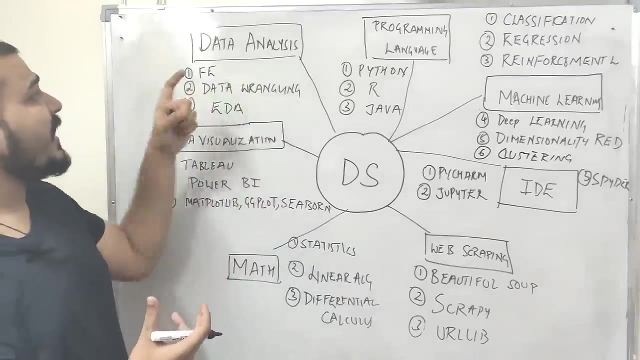 normal distribution, whether it has standard normal distribution. can i convert that into standard normal distribution? you know whether i have outliers in that particular data, whether the data is balanced, whether there are a lot of things that you can basically rule. uh, you know, take out more information from that particular data. now the main stage is this particular data analysis. now, 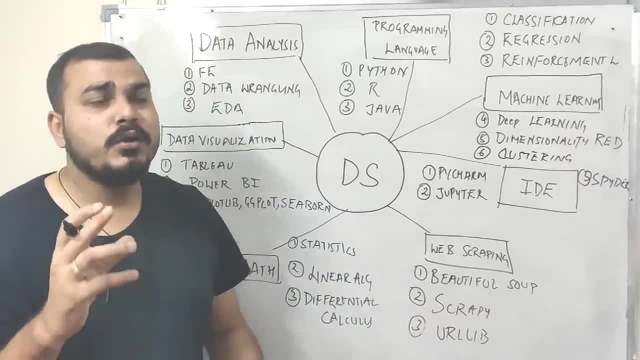 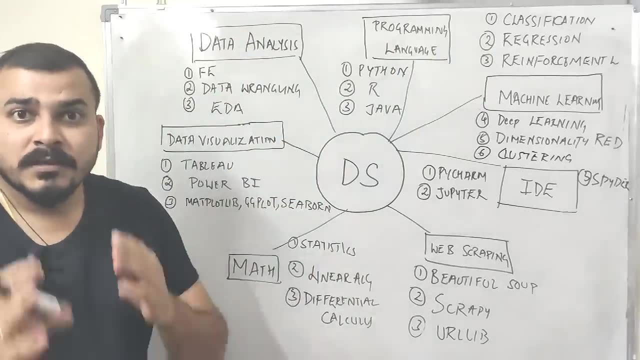 understand, guys. i have a use case. when you do one or two use case considering all these particular stages in mind, right, it is not like you have to study everything separately. take a use case, start solving it. i know many of them know python programming language, or our programming language. 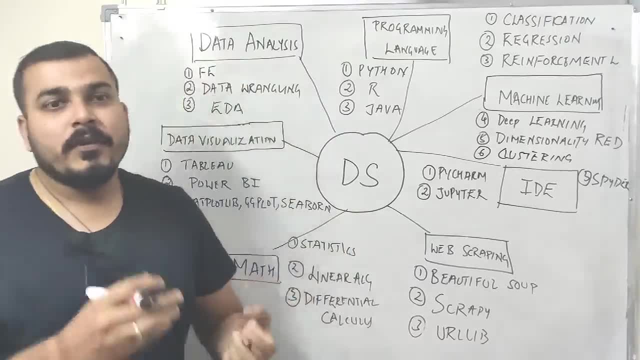 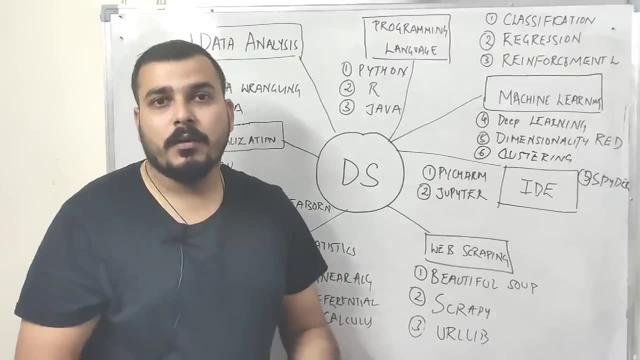 but you know- see an example- suppose i'm taking the house prediction right- what i'm going to do with that. first of all, i'll require data now. currently i don't have to do this, also because data is readily available. okay, for the first use case, since you're practicing, since you're making a 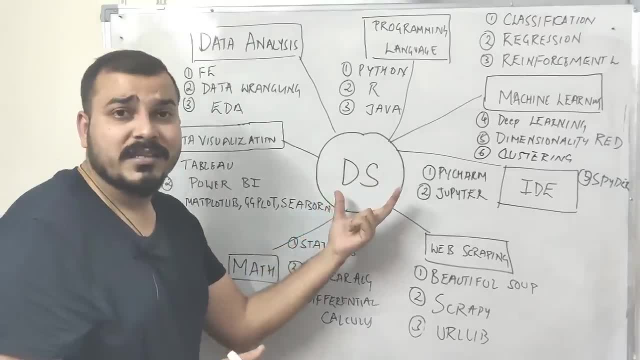 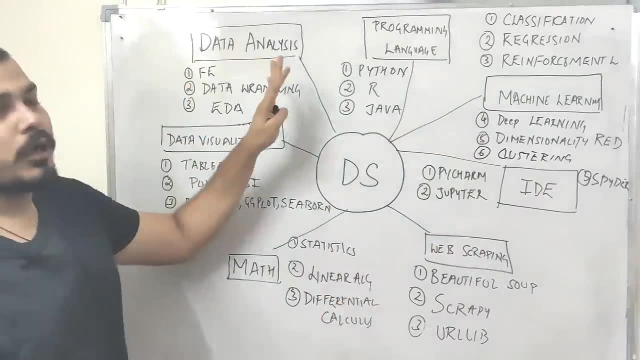 transition carrier towards data science, right. so for that, you take a use case, try to understand what that particular use case is all about. you know and then apply all these techniques whatever you require, and, as usual, the first technique that you will basically be applying is data analysis. 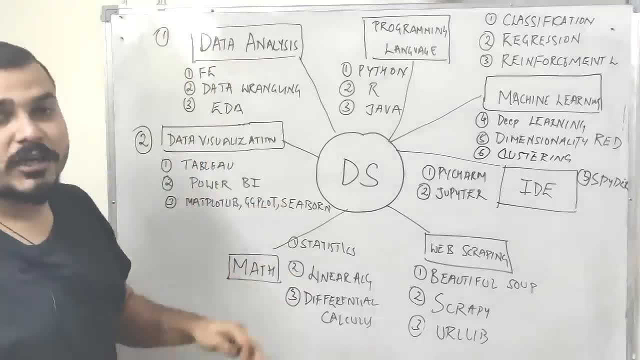 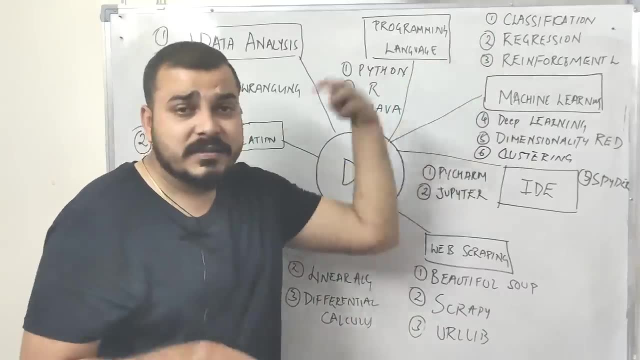 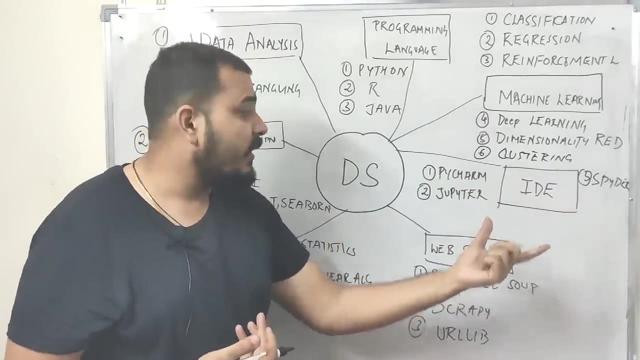 technique that you may do is that, after this data analysis, you'll also be utilizing the data to understand more about the data. and third thing is that you will basically be doing a machine learning algorithm selecting where, seeing that, whether it is a classification problem, regression problem, what algorithm you are going to apply, everything will be coming over here. 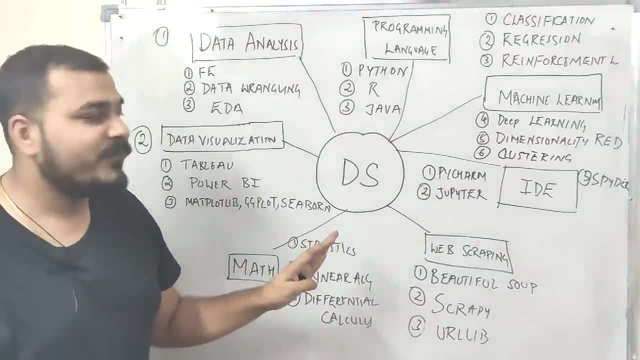 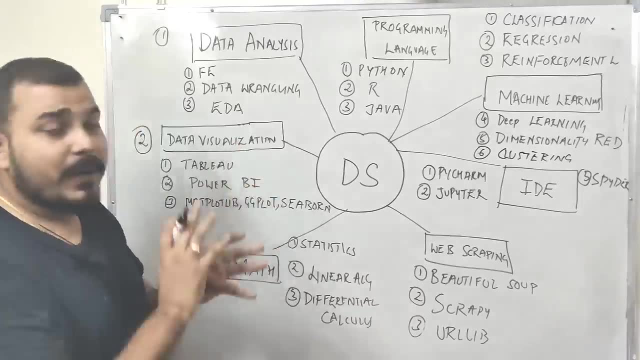 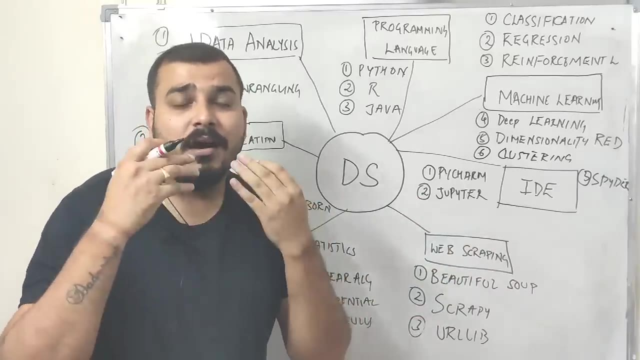 right, and then obviously you'll be selecting one id. that is for sure you'll be using pycharm, jupiter spider, so one of the best known ids for doing python, programming language or implementing any machine learning algorithm like that. so you know, if you, if you remember like, if even a lot of you know companies like 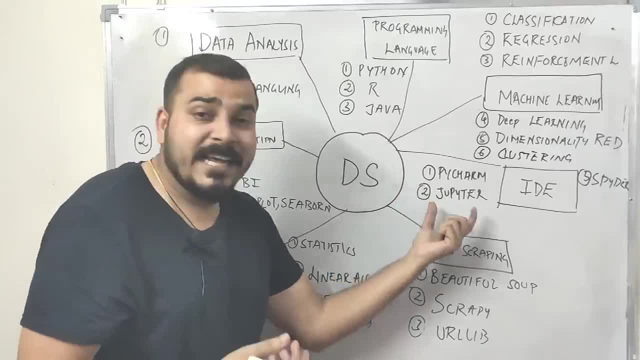 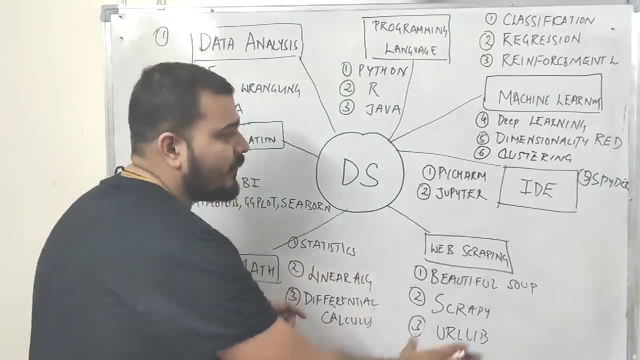 uh, amazon, which is basically aws, cloud azure are basically providing integrated jupiter id, so where you can basically code it and deploy it in directly into the production. again, deployment part is completely different from this deployment part. you'll have one more scenario where this will be with respect to your deployment. 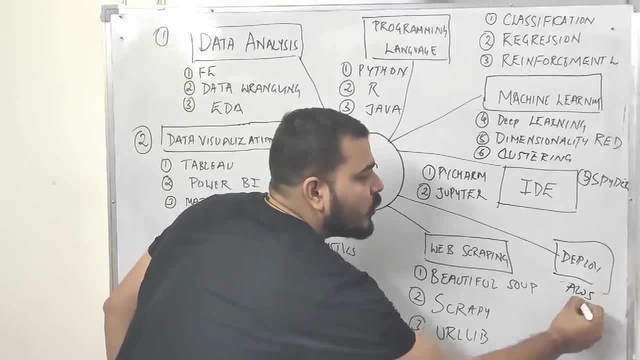 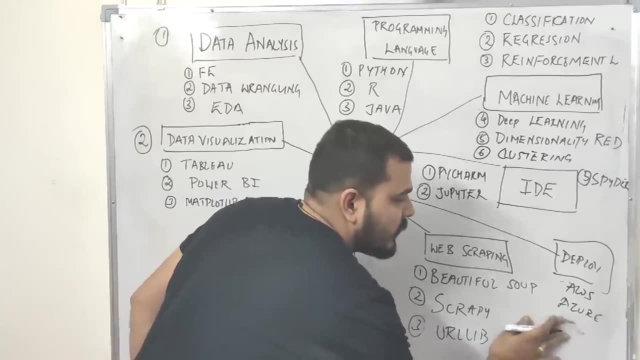 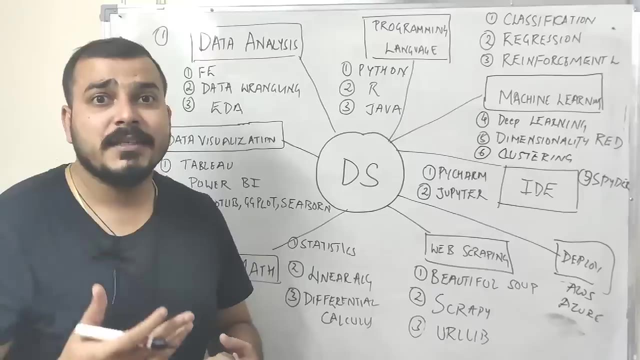 okay, now, in this particular deployment, what you are going to use is basically different, different tools like aws, or you may also use spark- sorry, it should not be spark, because spark comes into big data. so AWS, Azure, you may basically use some, suppose. if I take an example of AWS, you may take a ec2 instance and deploy a flask model over. 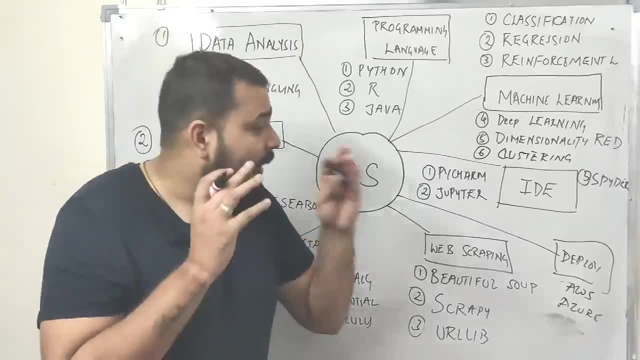 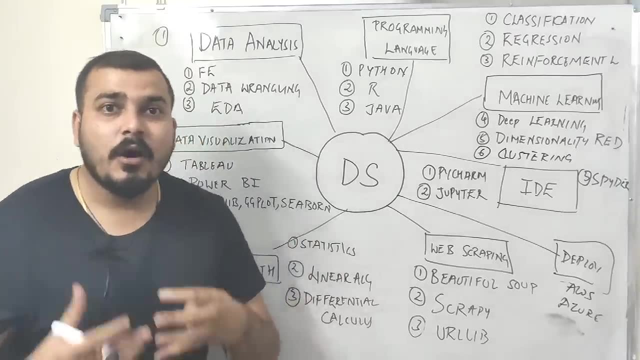 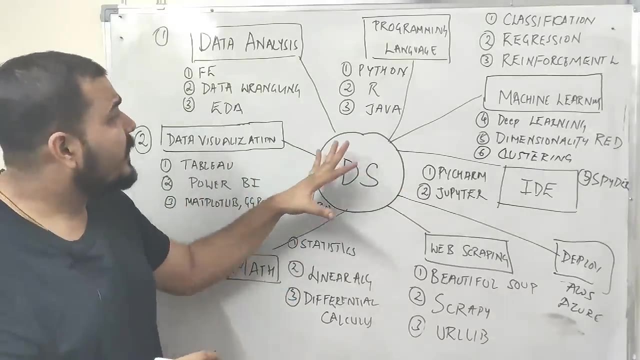 there. right, you should actually integrate your model with a flask framework and try to upload it in the AWS and create an API so that it can be consumed in the front-end. so how did I study? how did I learn? first of all, I took a very basic use case, as, as I took the use case right, I was basically you. 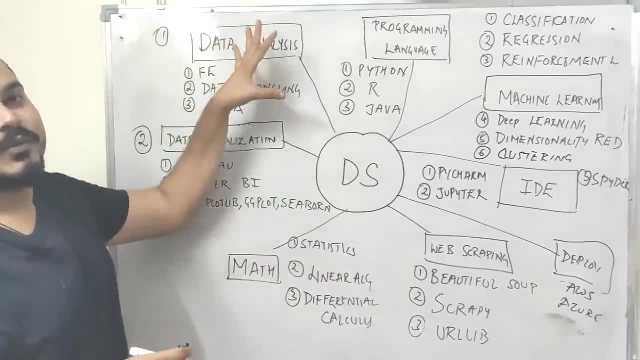 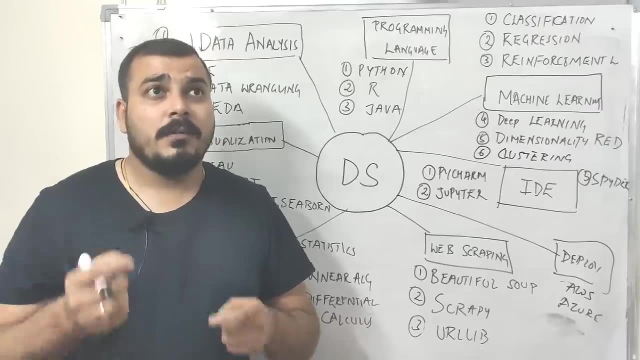 know reverse engineering, each and every steps of this, how the data analysis was done. so let me just remind you that one of the use case was already done regarding house price prediction and that was freely available. okay, first use case that I did was with respect to iris data set: iris data set. so basically, we 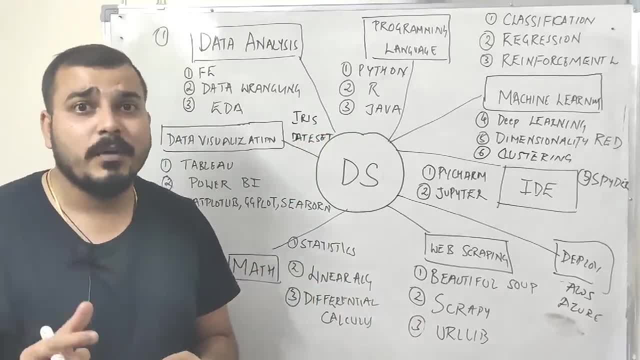 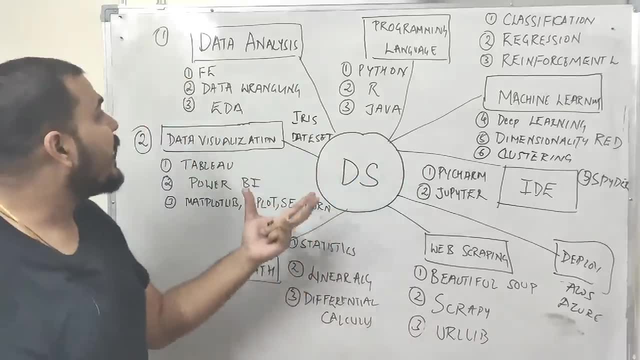 need to classify what kind of iris flower that is based on the sepal length and sepal width. okay, and this particular data set. the solution was clearly given in the internet itself. then I explored it, done reverse engineering? did the data analysis part? did the visualization part? 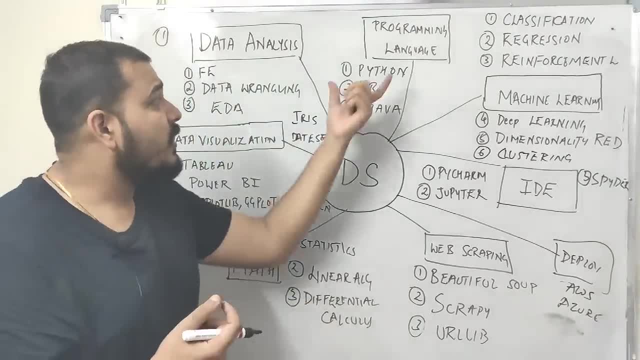 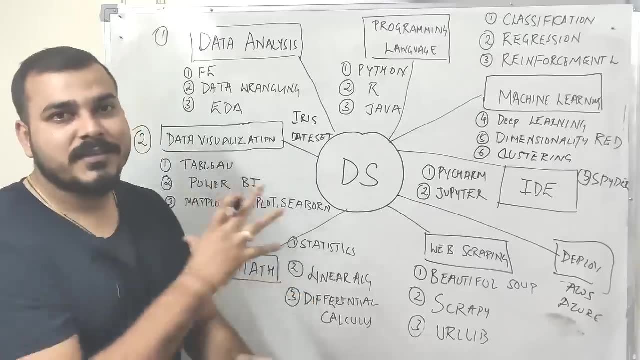 came to know a lot of things, okay, and initially when I was learning Python. also, you should remember that I was not perfect in pandas, using pandas numpy at all. it is all through reverse engineering that I focused. I try to understand the subject more, much more properly. I got more and more knowledge. 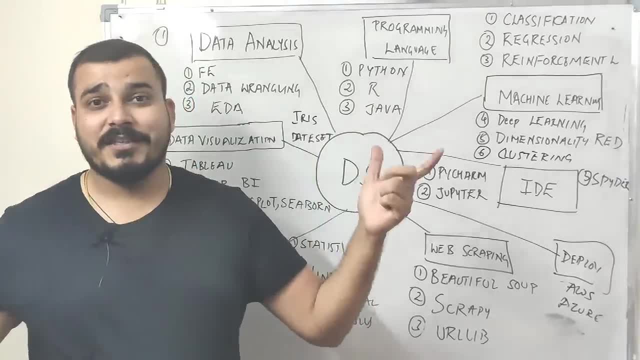 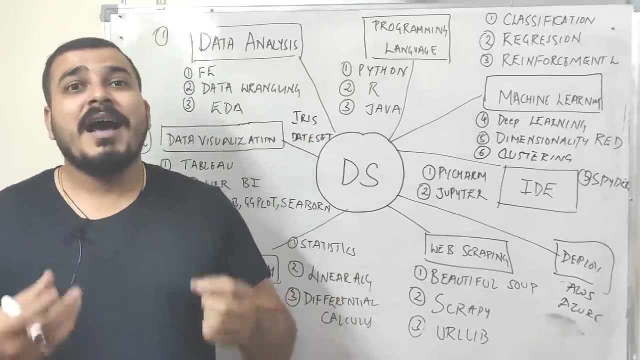 now, when you do reverse engineering also, you will be able to understand a lot of stuffs now. one example of reverse engineering is that if you want to clarify your environment, a lot of stuff is hard to clarify, but if you are having a lot of gym and reliability issues in your environment, this is popular. 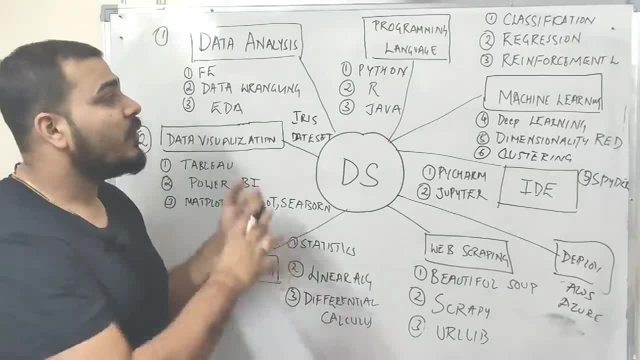 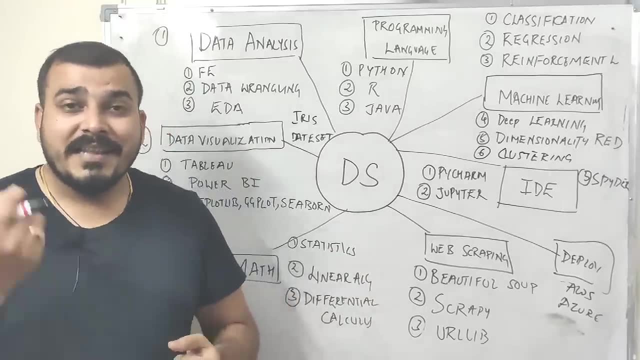 query or lawyers or collaborators. you should have this review and you should also cut down on zit based on the common weight orFS that you should have anyway. the other thing that I also loved was I couldening a few words about keep mirror serves. a brand of end-to-end do is open end users to. 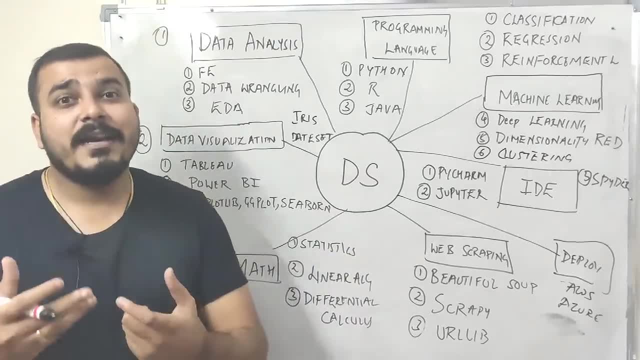 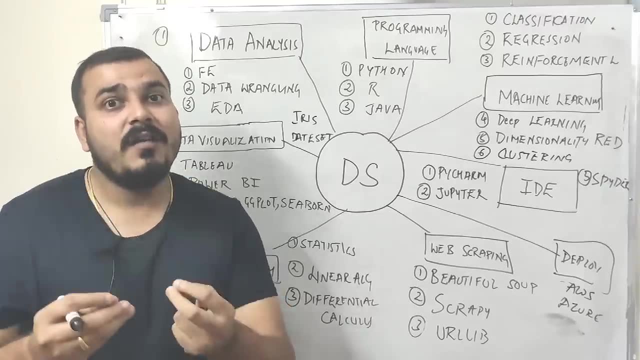 analyze new servers, which I think is great at home. obviously I'm smart enough if I'm not sure that art would work on many. even your managers will actually appreciate that particular work because you're able to give them. you're trying to solve a particular problem with. 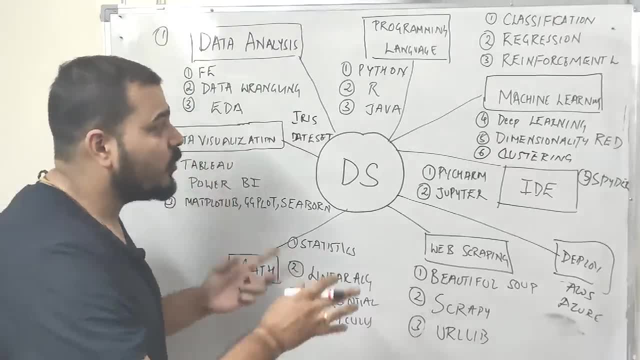 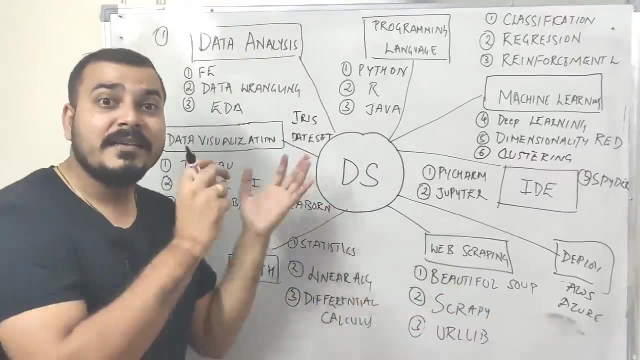 through the machine learning techniques itself. okay, so this is how you have to go. you have to basically do a reverse engineering. try to follow this pattern. see the use case. it is not like every project can be created like a data science project. understand a use case and based on that use case can you solve. 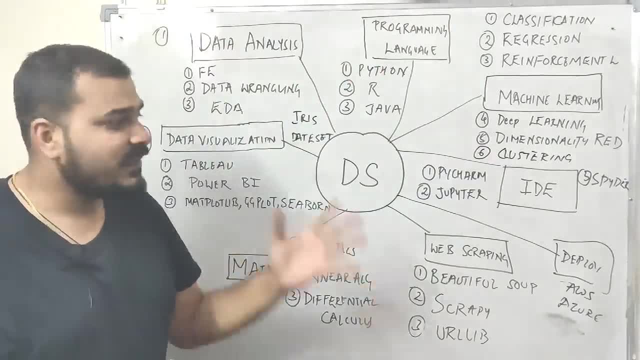 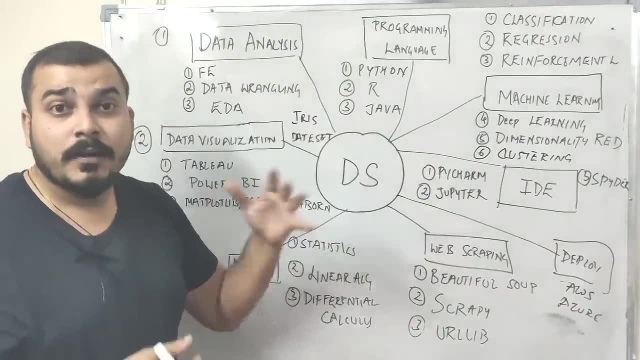 the problem and for that, what are the steps that you're basically going to apply? and this is the whole diagram that I have drawn in front of you. I've included everything and you have to become perfection. you have to bring some perfection based on the reverse engineering that you're doing in various 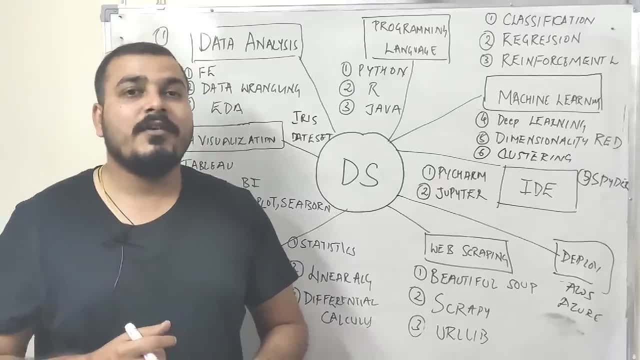 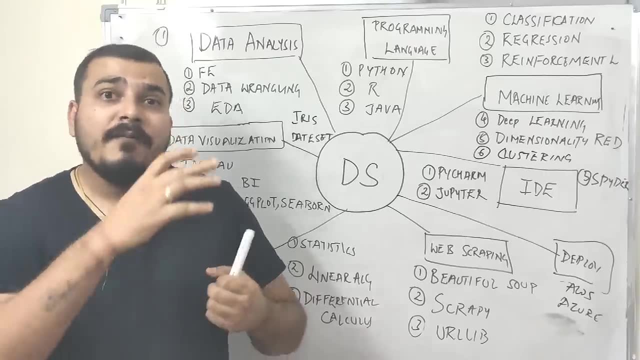 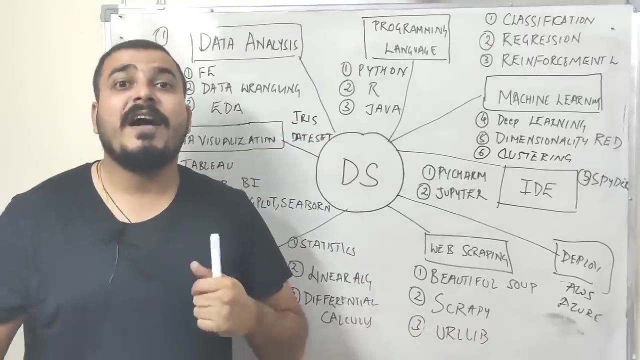 things. okay, let me just give you one more example. so for the first time when I was handling category feature, I just used to know about one hot encoding. okay, now, later on, I got scenarios wherein I have many category features and if I was performing a one hot encoding, it was unnecessary creating so many columns. so 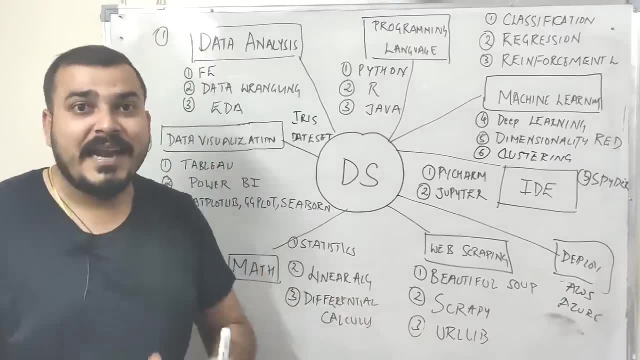 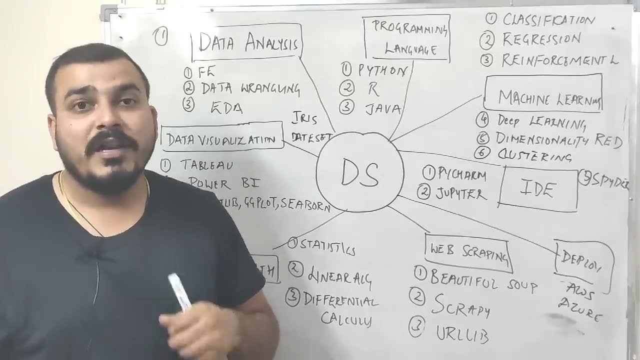 I found out a different way how to handle that scenario and, as I said that it is with all reverse engineering, I was based, I was basically doing a use case and that problem came at that particular point of time. so I thought: how could I solve this? I did a. 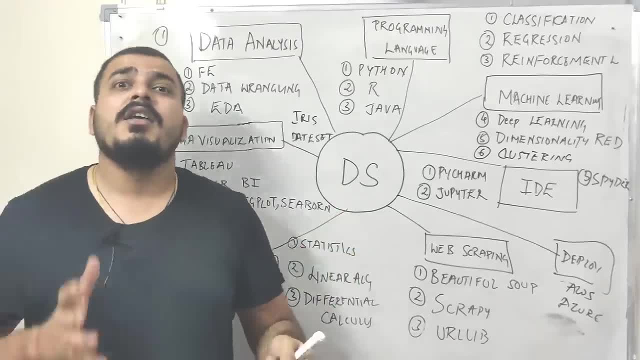 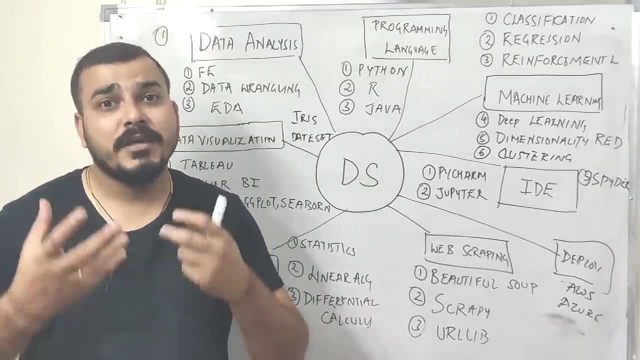 lot of research and finally got a lot of inputs from the data science community. you can handle this like this. there are a lot of competitions that was done. I saw Kaggle competition. I checked out kernels that was freely available and I was able to get in their knowledge. okay, and that is how you have to do reverse.